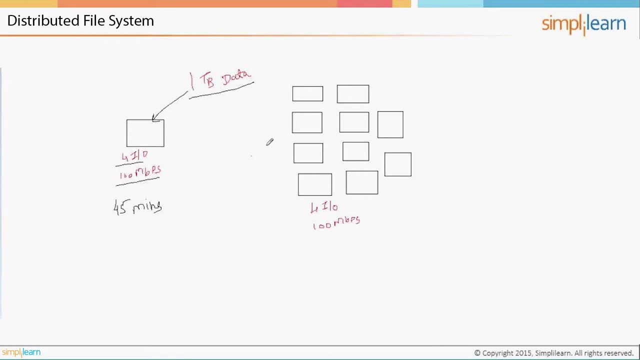 then, of equal capacity. by the way, each machine will have four IO channels and 100 Mbps speed. Now they are distributing this one terabyte of data into multiple physical machines. You can see it like that, So and so on and so forth. So some part of the data is stored. 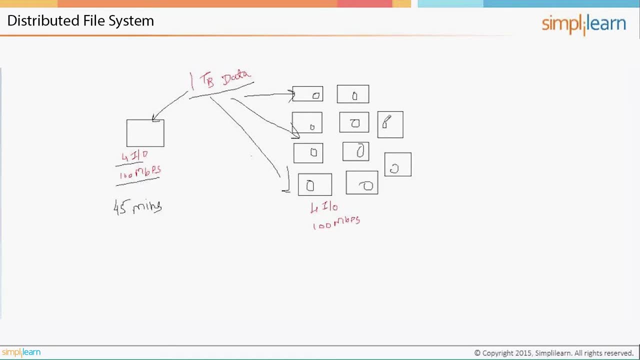 in one machine, some part of the data is stored in another machine, and so on and so forth. Now, if I want to process this one terabyte of data which is distributed in 10 different machines, I can parallelly do that processing. 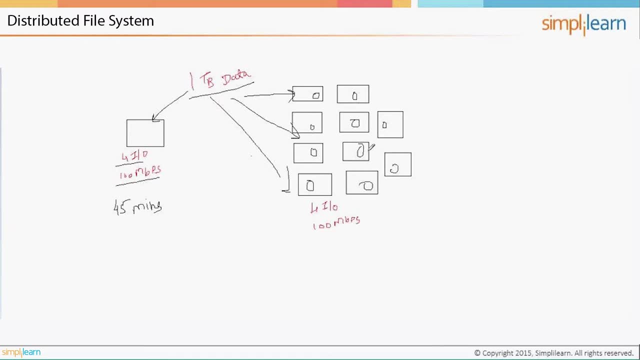 So how much time I can, how much time it takes to process this data from this 10 machines in a parallel manner. So it would take approximately 4.5 minutes, Considering we are not considering any network transfer, network latency and all that which. 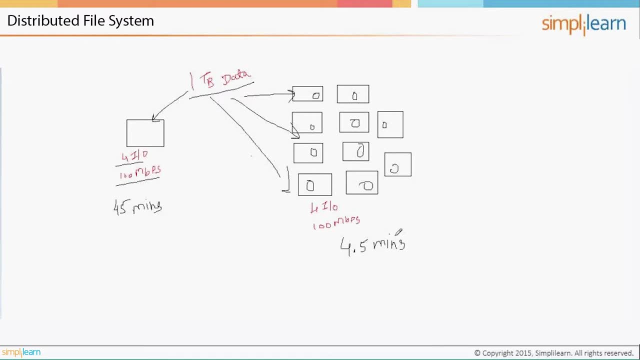 will be not very huge. So approximately it comes to 4.5 minutes. So what I am trying to highlight a point is, if you distribute your data, You can get parallel processing advantage and you can perform 10 times better than this older systems, right earlier case. so that is. 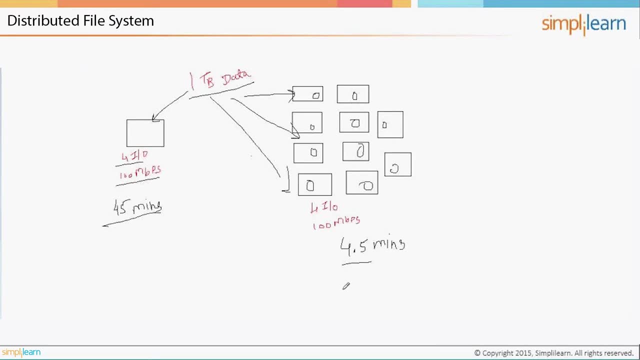 the fundamental advantage distributed file system provides. there are lot of other advantages it provides and we will spend lot more time on understanding the entire HDFS architecture. how does it store data, how does it process it, how does it do the failures and recovery and all that stuff. but right now let us understand this important part, which is by storing data in a 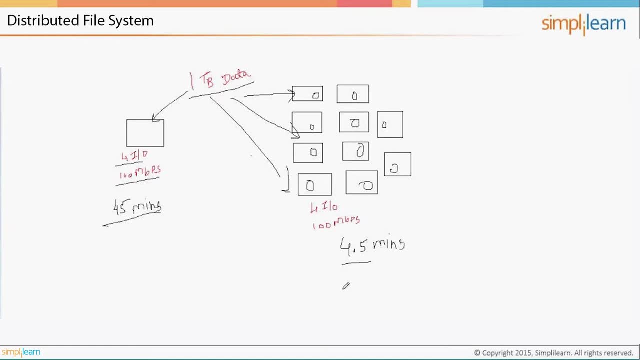 distributed manner in different machines, you will get an advantage of processing them in a parallel manner, increase your performance and decrease the processing time. that's a fundamental reason why DFS came into existence: distributed file system. now let us understand what is DFS. what is distributed file system? very, very important to understand this concept. if you understand this, you understand as DFS okay. 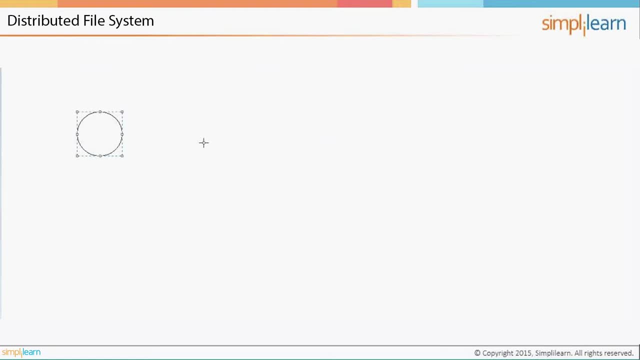 of course there are a lot of details you need to understand, but if you understand this stuff, which I am going to explain right now, at least your basics of distributed file system is clear. so let us assume that there are four physical machines here, okay, and each of this machine? 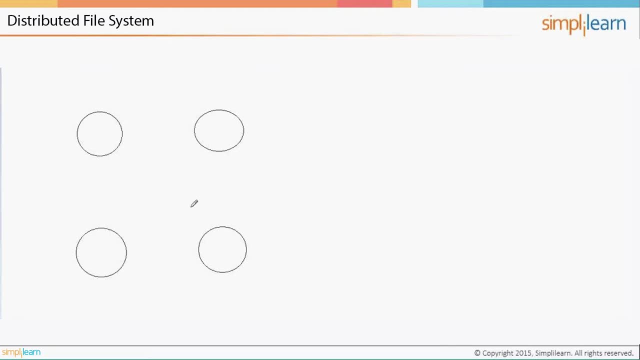 is connected to a DFS and each of these machines is connected to a DFS, so let us assume that there over a network, we just highlight it this way. so if they are, they are connected here, or a network, everybody is connected to everyone else, right? this is part of one organization. it may be possible. 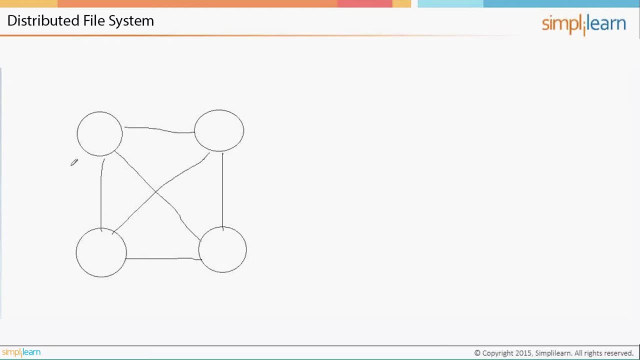 that one machine is in one geographical location, another machine is in another geographical location. that is possible, but they are connected over a network. now, when we talk about one physical machine- and for that matter, even your laptop can be one machine- right can be considered as one machine. so each machine will have its own. 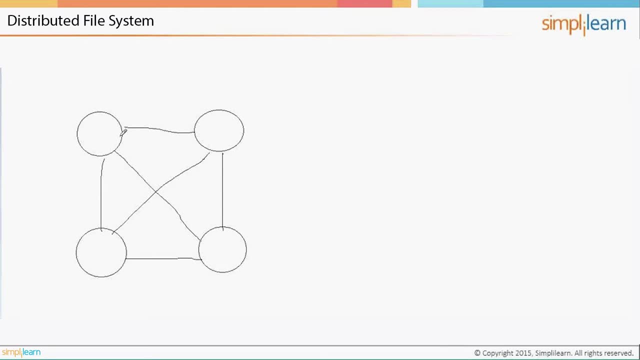 local file system or a physical file system where you store data right where you create files and folders. normally in windows you have c drive, d drive, where you create those files and folders. internet uses those you know NFS file system and and then basically stores that. but anyway, we will. 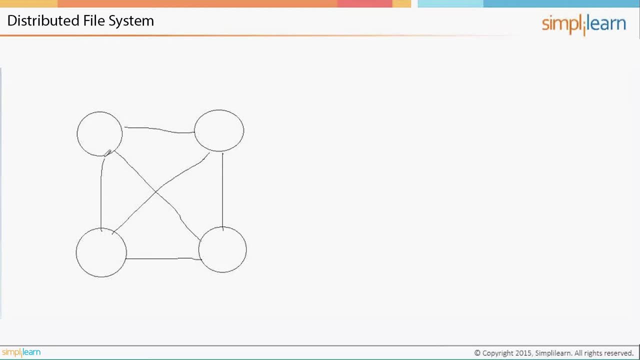 will consider that as a file system, so that's a local physical file system. in linux or mac you have slash, home, slash, user directories under which you go and create your own folders and directories and files. so these are all local file system which is available for every physical machine. 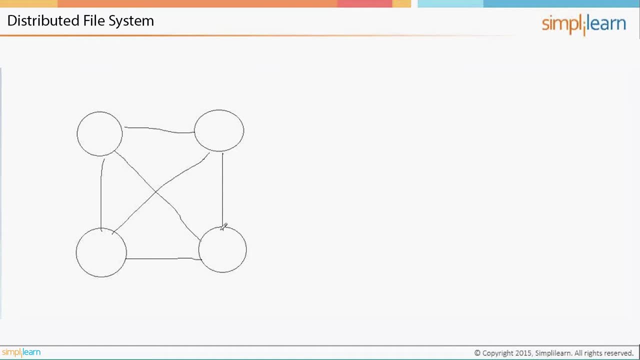 right. what is a distributed file system? distributed file system is actually. see in in this name distributed file system, you have something called file system, right? so whenever we talk about any file system, you can easily assume your. you know in in case of windows you can assume your c drive, d drive kind of file system which where you can go and browse. 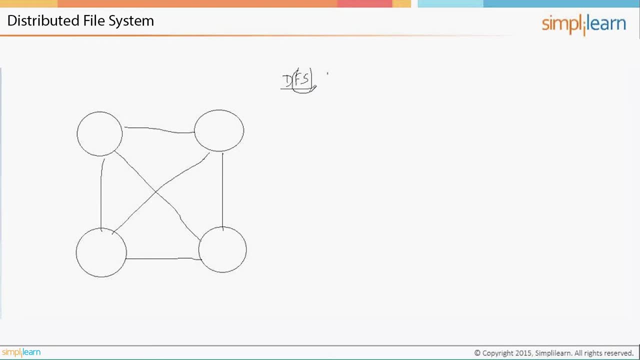 any folders go inside that explore different files and all that stuff. but the moment you say distribute it, it's not physical. okay, so any distributed file system is actually not physical file system. it is called virtual file system. so let us understand this part little bit more. when i'm 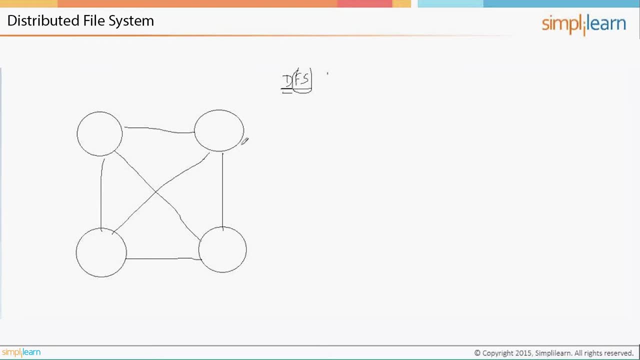 installing hadoop. now i'm talking in terms of in the context of Hadoop. Why? Because, of course, we are going to work on that for a longer period. So Hadoop uses SDFS, which is a Hadoop distributed file system, right? So whenever you want to install Hadoop on 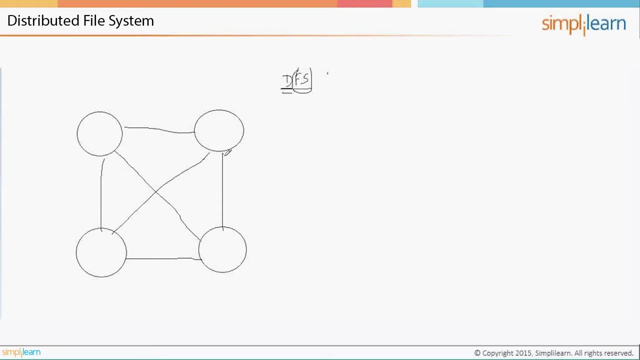 any machine. let's say you want to make one cluster. I think somebody has a question. initially, what is this cluster? Cluster is nothing, but it's a set of machines connected over a network. So this, this, this and this, these four machines are connected over a network. So that becomes: 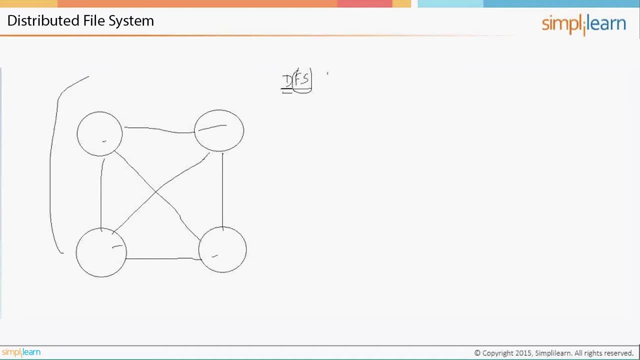 one cluster. Okay, That's how we can refer a particular cluster. All right, So they are connected over here over the network And we are. we understood that much. Now, we were talking about the distributed file system, So basically it's a virtual file system. Now how do we? 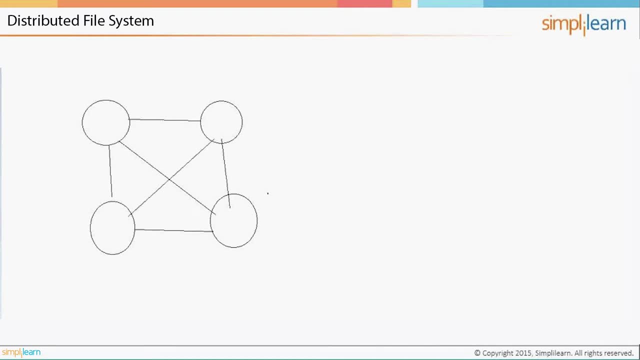 understand whether what is virtual file system. So we all understood that every machine will have its own physical file system. So whenever you want to install Hadoop, let's say you want to install certain libraries of Hadoop in every machine, right? Ultimately it's a software. 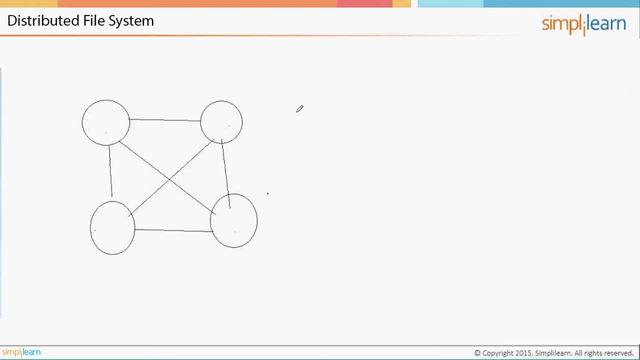 So we need some libraries and some programs which needs to be installed in these machines, And then we need to start them And then we we will say that yes, we have installed the entire Hadoop cluster right. So let's assume I have installed certain programs in this machine, certain programs. 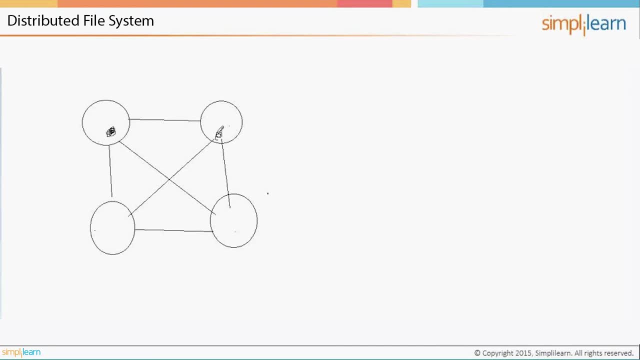 in this machine certain programs here and certain programs here, Okay, Of Hadoop, And all of these are in, in, in in their own, you know environment. So normally entire Hadoop is written in Java. So these are all Java processes. They are running in a separate JVNs in different machines. 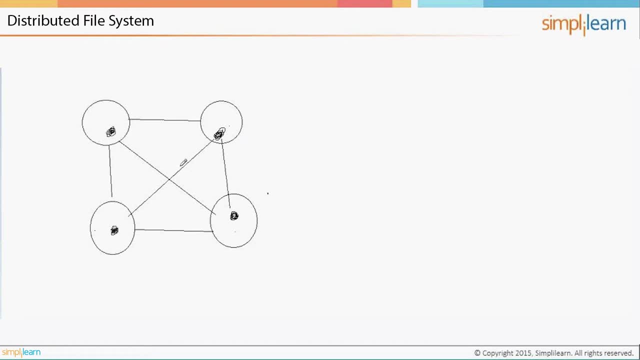 They are actually creating one virtual layer which comprises of all the physical machines underneath- Okay, This virtual layers is called DFS- distributed file system. Okay, Now what happens? Let's understand. Let's say you have a file, Okay, Which is having one terabyte size. 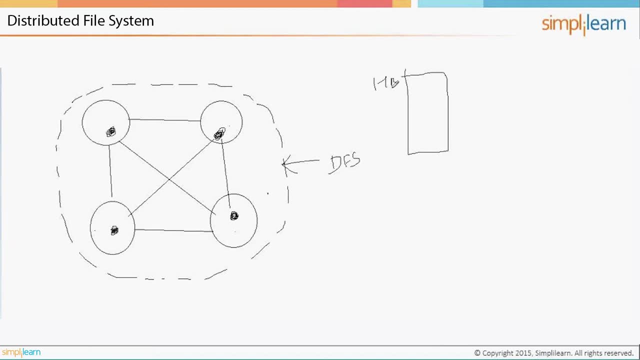 I have a file of one terabyte size and I want to store this file name is, let's say, F1. And I want to store this file in this distributed file system. So normally a distributed file system is again is called DFS, Is called DFS. 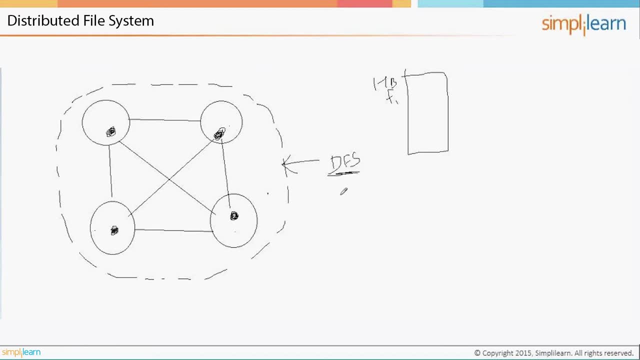 It's a virtual file system, It's a set of programs, It's a software. So obviously it will have its own command which we can use that command to store data in distributed file system. So I can, as a user, I can use some commands. 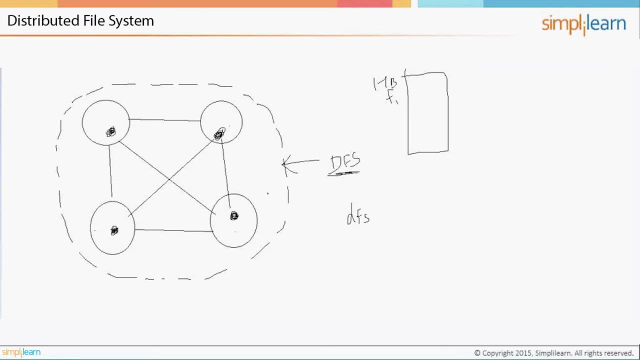 Let's not worry about what command I'm using. I'll just say DFS, F1 copy. I'll just say source location and destination location. This is the command I'm going to write. The source location is the location of the file, where it actually belongs right now, And the destination path is a location where I'm going to copy that file. Let's say I'm creating a directory name data under root directory and under which I'm going to create this file, Ftxt. 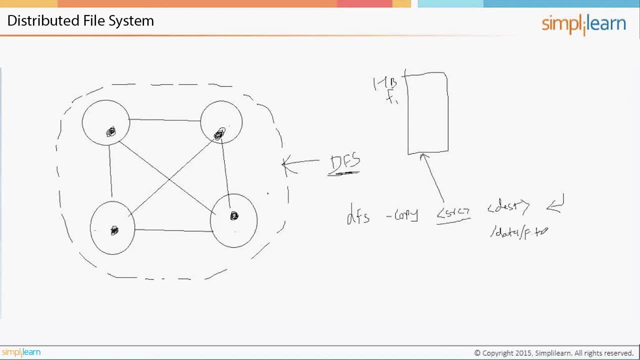 Okay, Okay, When you execute this command, this entire command is a user. what happens behind the scenes, these programs which are running and which makes up this entire DFS? they will what they will do. they will first go to this source location and pick up this file divided into multiple parts- a, B, C. 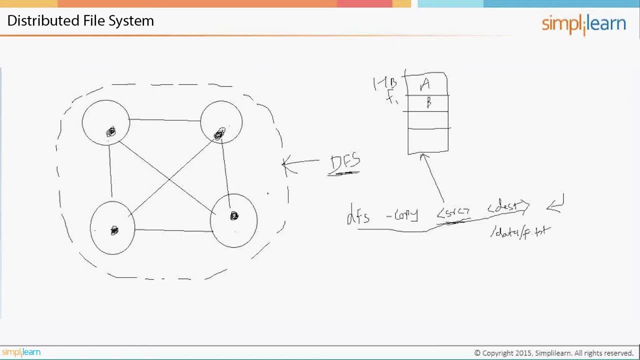 and D and each of this part. they will store it in different, different machine: a, B, C and D, like that. okay, this is completely transparent to the user. user is not aware whether it's file is actually physically divided into four sub file. this is also file. these parts are nothing but small files only, which 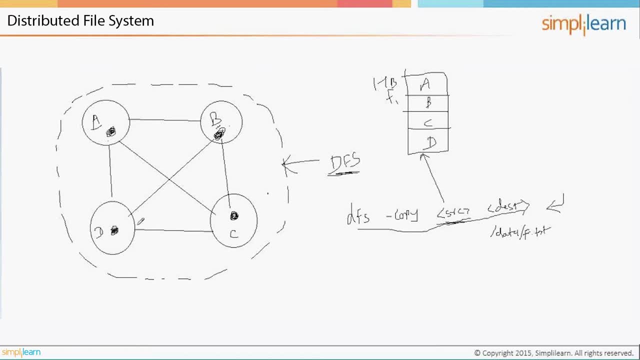 contains partial data of the original file. okay for us as a user. we think that we have stored everything in this particular path in this location, but actually, behind the scenes, it's distributed in multiple physical machine right now. when you want to read that this, what is this path then? where it is present? this path is not present. 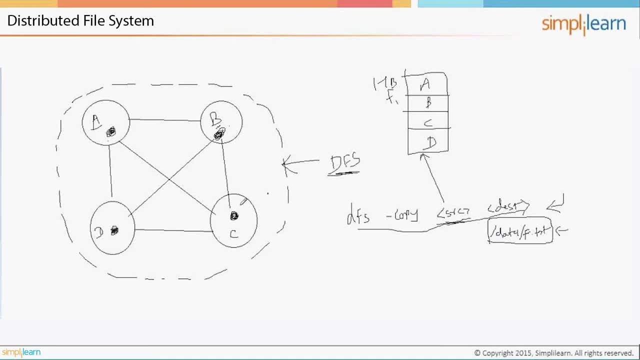 in any of this machine. this is just a virtual path and it is remembered as a metadata information. that's it. so when you want to read it as a user, I will just refer this path. I'll just say DFS, I fun cat and I'll give this path. this is. 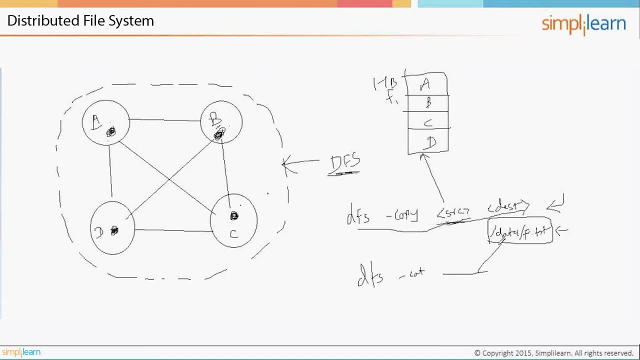 the path. I will put it here. and when I execute this command, I am thinking that I'm going to read that entire one terabyte of data from a single machine, from this path. but behind the scenes, what happens again? these programs, which already remembers that your file is divided into these many blocks. they also 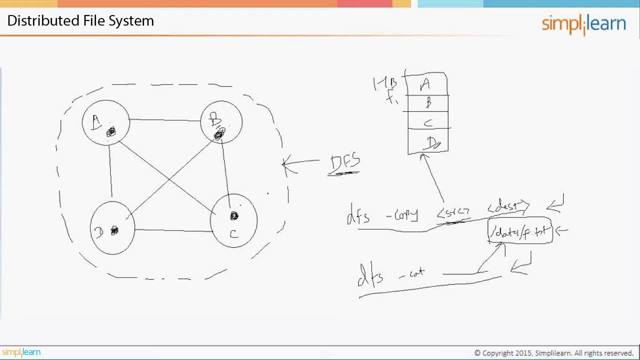 remember the location of every blocks in this machines. so it goes, reads every block in that order right and preserves the data to the user. this way again it's complete transfer and to the user. so that is how distributed file system works. so it basically, when you store data in DFS, we think that it's a physical file system. 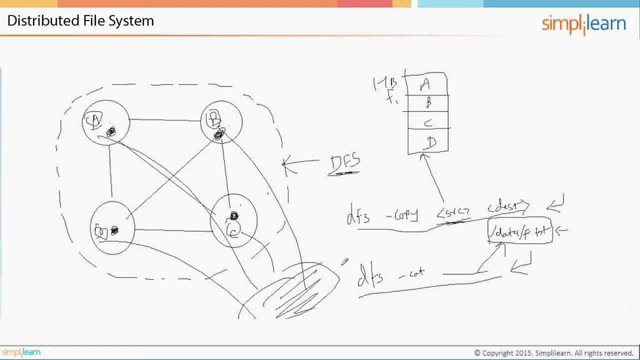 and we have loaded in in this physical location. but this location does not present in any machine, it is just virtual location. physically, the data gets distributed in multiple machines behind the scenes and then when we read it again, it will go and read all the data from those machines and give you. 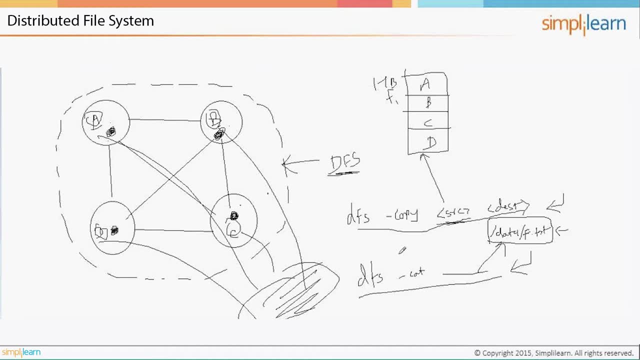 the data. that is what we're going to show you in the next video. so, thank you. that is what we mean by DFS. ok, one more disclaimer here. I have just given you a high-level ID on DFS and virtual file system. we did not understand the architecture. we don't know who is controlling this information. 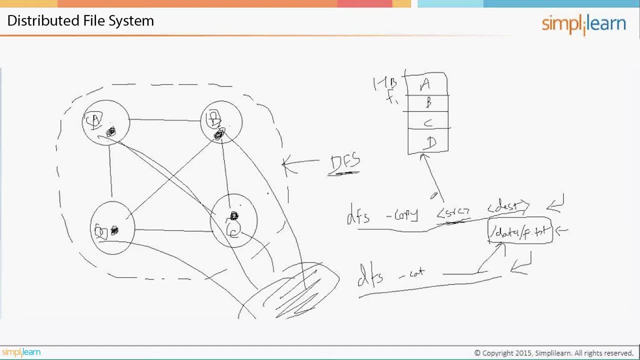 whether there is any server or not, whether there will be any master or not where this metadata information will be present. what happens in case of one of the machine gets failed? there are a lot of stuff that we need to understand and are going to do it in coming up sessions, but i am going it step by step, where i am just explaining. 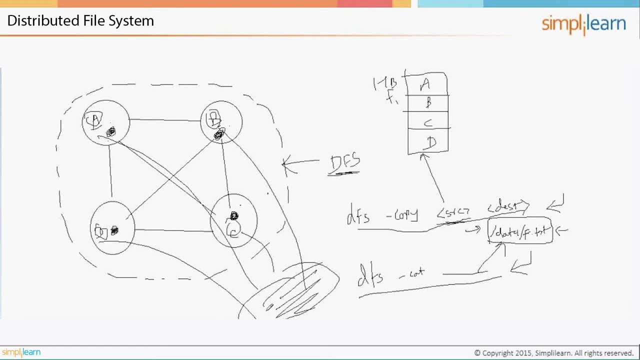 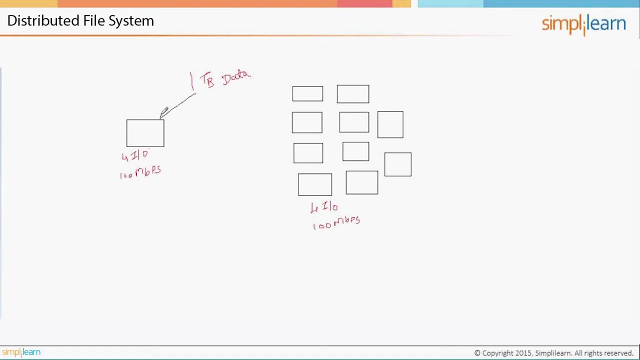 you some high level details so that you get familiar with that term, right? so why dfs? uh, because, let me, we just discussed, right, that i have one physical machine. if i store all one terabyte of data in that machine and if i want to process one terabyte in a single machine, it will take. 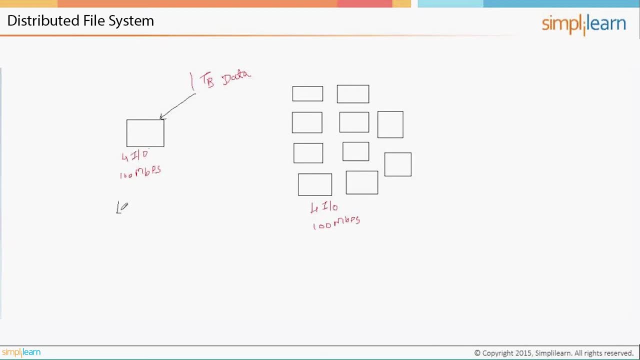 about 45 minutes of time to do that. but if the same data, if i distribute it in multiple machines, right, using a distributed file system, just the way we understood just now, uh, and then i can actually get a chance to parallely process all the individual parts of this file, right, so i can. 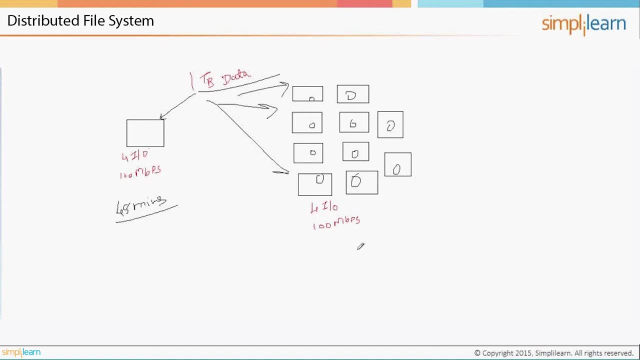 process this one terabyte of data in 10 times faster time than the original use case here. so that is the fundamental reason why dfs is necessary needed because you can process that, because you can store the data in a distributed manner. you can increase it parallely. you can process it parallely. 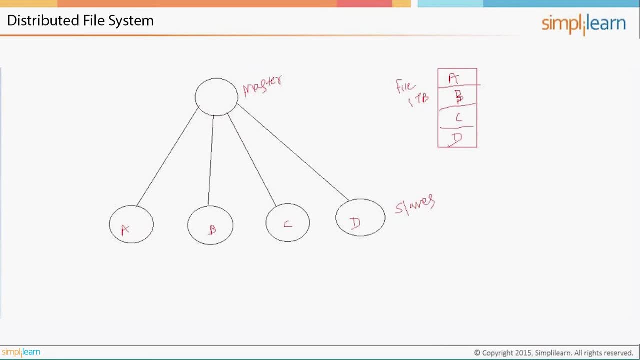 okay, so any distributed file system is a master slave architecture, by the way. so we are going slowly towards you know, uh, very close to what hadoop looks like. so this is called one cluster, cluster of five machines. one machine is master, others are slave. okay, here, uh, a master. as you can see, here i have stored one terabyte of file, so all the parts. 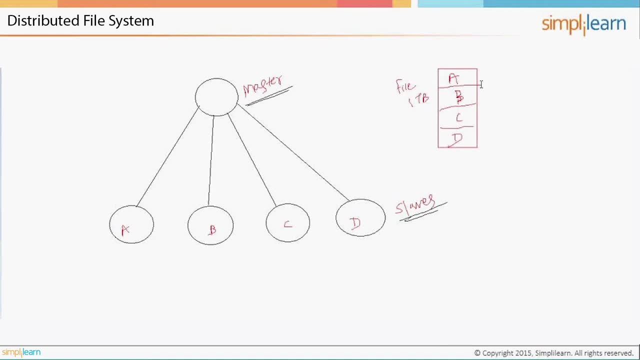 of the file are stored in slave machines. master does not store any data, so in any distributed file system master will just remember the metadata. that means file to block mapping and block to slave node mapping. which block is there with with slave node machine? this is called metadata information. okay, this is slave node one. slave node two. slave node three. 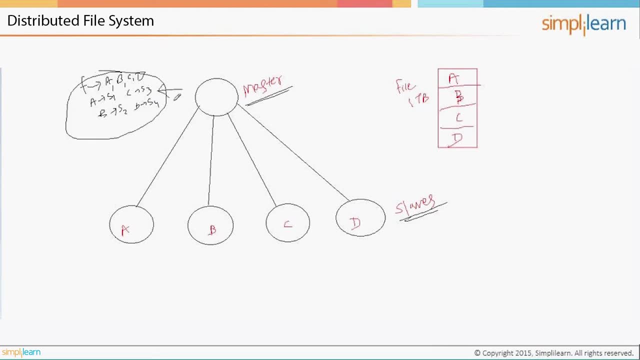 slave, node four, and so on, so forth. right, so master will remember file to block and block to location mapping. that's the metadata which is there with master for all the data that you store on as on on a distributed file system. slave will just remember the x will store the actual data. 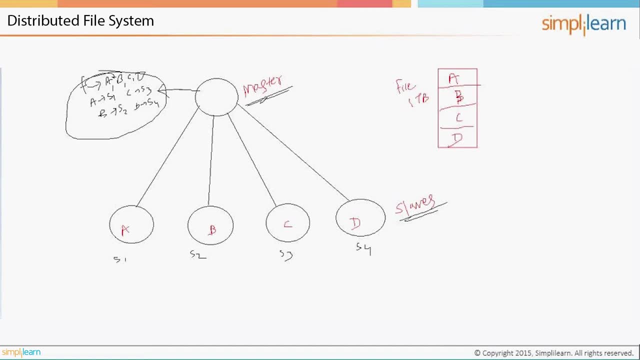 so this is called metadata information. okay, this is slave node one, slave node two: slave node three: okay, so that means master becomes one of the very important process in this cluster. who remembers the metadata and any client who wants to access the data will have to go through master only. 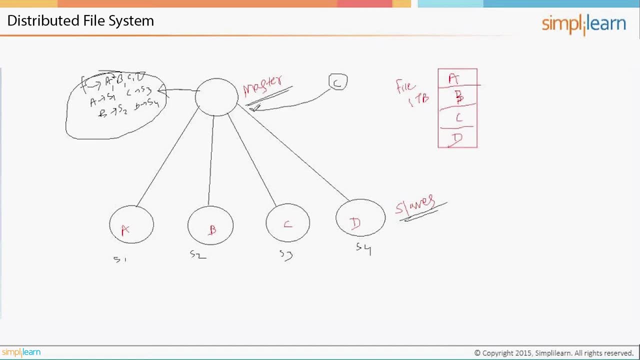 to access that data right. so that's why master becomes very important. there is no other way you can access data except routing through master, because master only will get you the exact location where you can go and read the data or access the data right. master actually is a very, very important process, and we will also cover the scenarios like when: 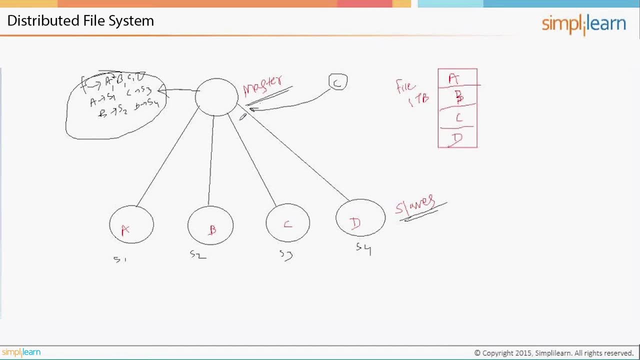 master fails, what happens? how to take up the backup of masters, how to take a backup of all this metadata. all these things are going to be discussed in the architecture that i'm going to cover on sdfs, but right now we will just understand. first, high level differences between hadoop and 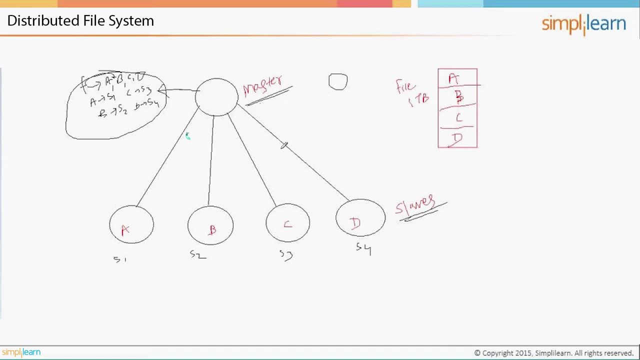 traditional system. so, yeah, this is how the any distributed file system looks like, and for that, even hadoop is also having the same architecture: master slave architecture. now assume that there is a client who wants to read a file. he will go to the master, because master knows the metadata, and then master will tell him that this 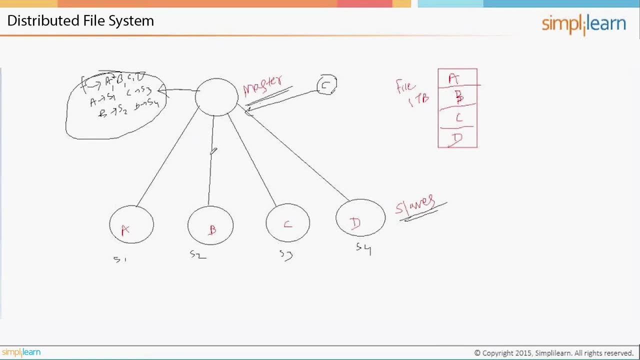 file has four blocks so you can go and read it from this four machine and client will start reading it from them. now, during the process, when it is reading the data, one of the machine fails. if that machine fails, client will not be able to read one of one part of the file, right? so what does that mean? that means client will get a partial. 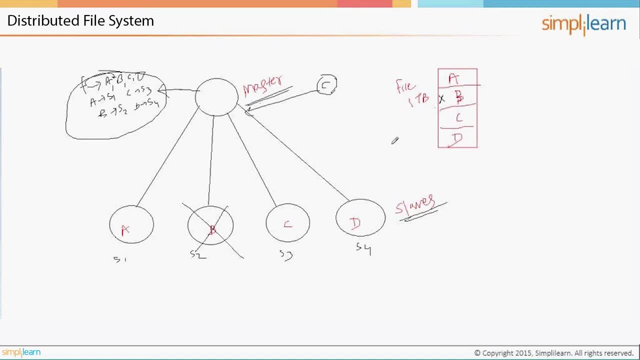 data. so that is a problem. so during any failure of the node, when we say node, node is nothing but a single machine, single physical machine in the cluster. so any machine in the cluster is referred as one node. so if one of the machine or node fails then client is not able to access data. 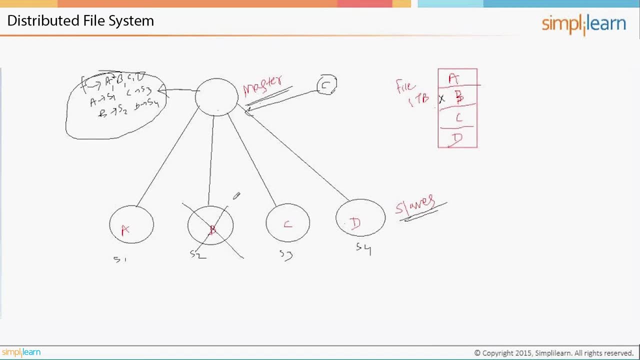 stored on that machine. so what distributed file system does they actually do that? they actually, you know, take care of this scenario by using a functionality called replication. replication factor is basically configured when you set up the distributed file system cluster. you can configure it as two or three or four, or 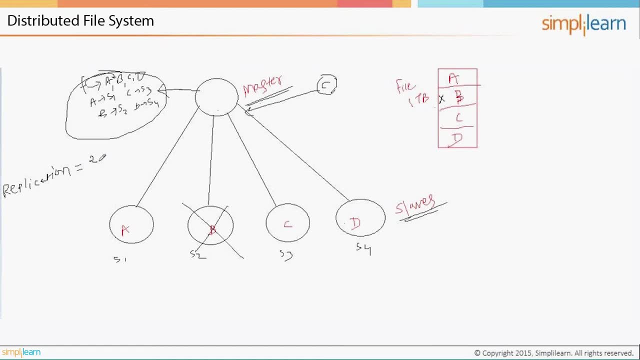 whatever, when you configure it as two, what happens? every block will be replicated two times in the cluster. okay, every block, every block will be replicated two times in the cluster. so what happens in this case? if one machine fails, i can still read one of the copy of part b from other available machine. right, and i can read the complete data. so, basically, 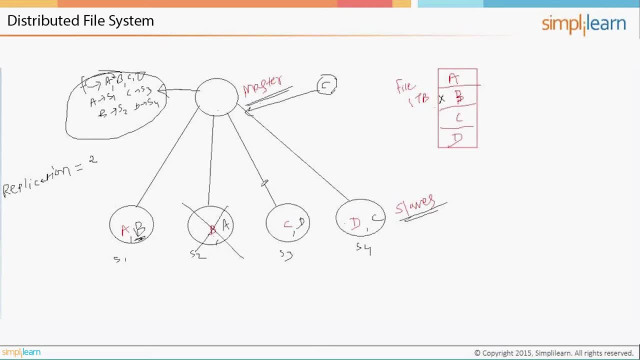 this is called high availability of the data. if one machine fails, i can read it from other machine also. this is called high availability of the data. okay, and that is guaranteed by some of the distributed file system, not all. Hadoop guarantees that traditional distributed file system like Teradata. 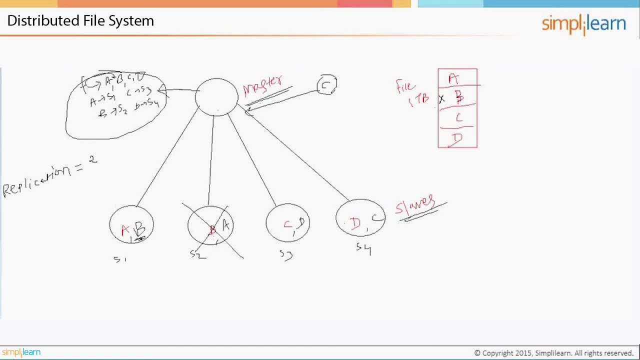 does not guarantee that, why? let me explain you that. okay, all right, so now I will actually tell you one important thing which not every distributed file system is giving you guarantee in terms of high availability of the data. so let's understand that point little bit in detail. so let me draw this first. 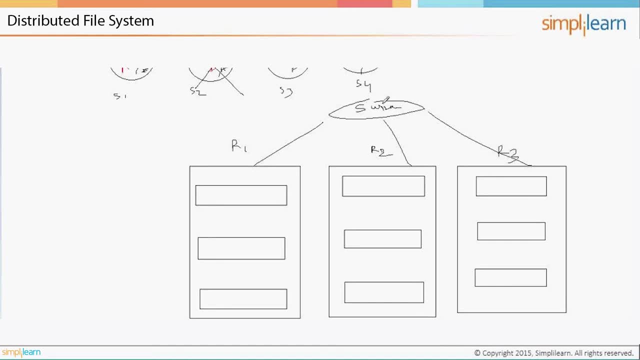 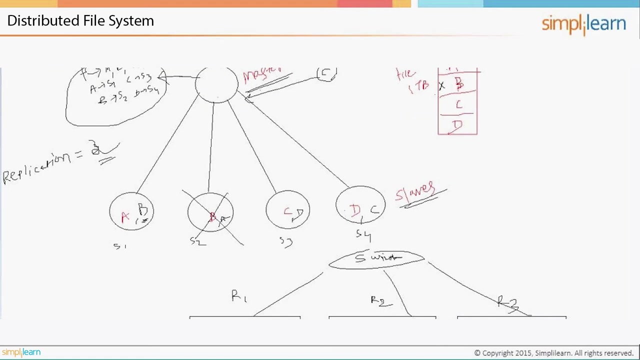 this is switch. pardon my writing. okay, now this is called REC. I'm sure you could have seen command center or data center in your. you could have seen command center or data center in your. so let me draw this first. you have seen the command center and data center in your company. you will see. 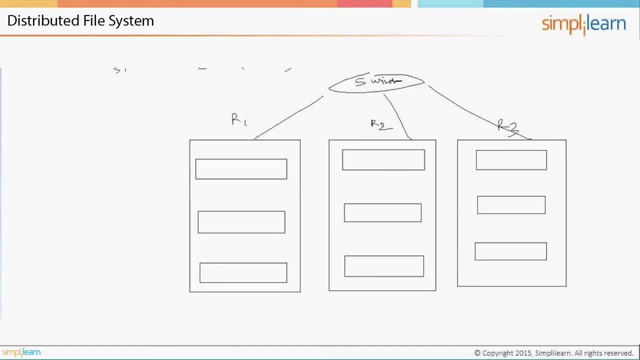 that every data center or Command Center will have lot of Rex installed right. so you'll have multiple ranks and each Rack will have its own machine physical machine. you have machine one, two, three, four, five, six, eight, nine and so and so forth. now each of the Rack will have this physical. 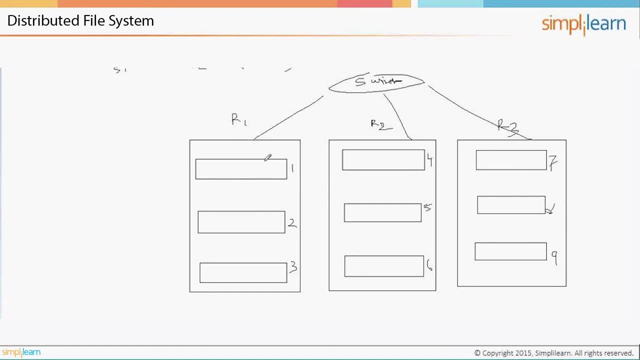 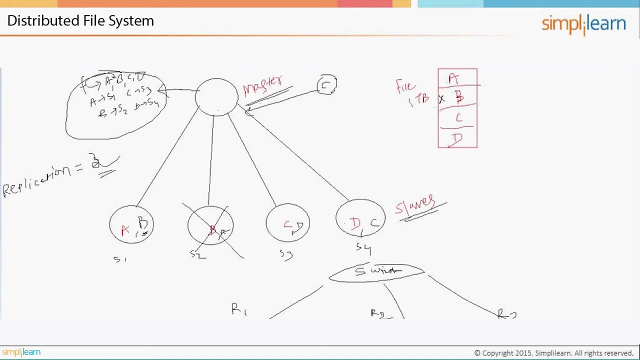 machines installed and they are connected over a switch to connect to the outer world. so basically, when you deploy a Hadoop cluster right, it will not look like this. this is just for your understanding. I have shown it in this way: master and slave. but actually physically, this is how a cluster can be. 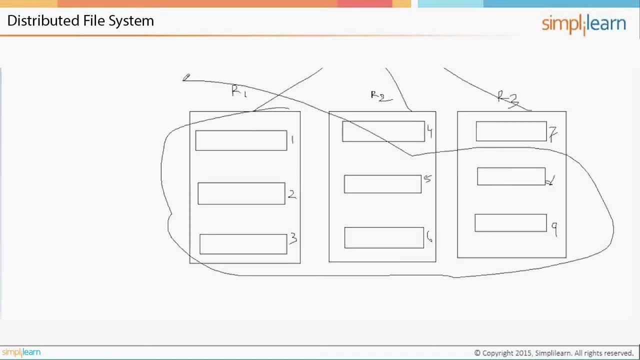 seen. all these nine machine together is referred as one cluster in which are which are installed in three different rack. each rack is, by the way, its own device and each device will have a space where you can install all these machines. one of them can be a master, others are all slaves. so let's say I have the same. 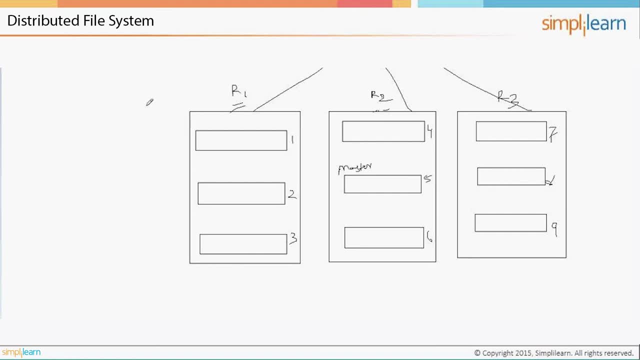 file. let's say I have a file which is divided into multiple blocks, ABC, and the application factor is 3. so first of all, let's assume that I am storing my data in this fashion. now, can you see any problem here if I store the data in this fashion? so 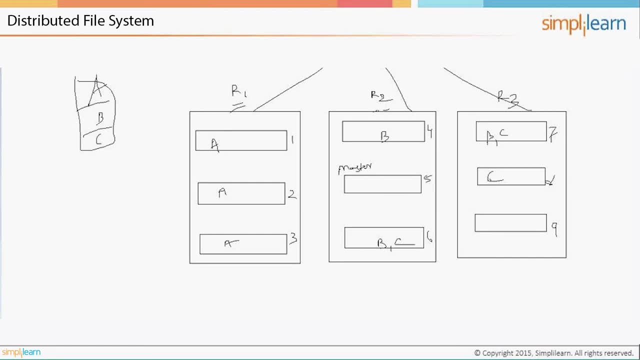 basically, if rack one fails, I will lose all the copies of block a, even though I have replicated it three times and stored it in three different machines. if my rack one itself is fail, I am still losing all the data. so this is a problem, and this problem was addressed by the machine itself. so this is a problem, and 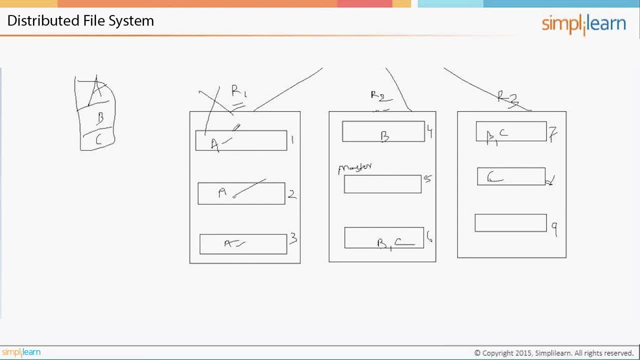 this problem was addressed by the machine itself. so this is a problem and in Hadoop, Hadoop always guarantees rack awareness, whereas traditional distributed system does not follow rack awareness. so we'll be understanding rack awareness later, but right now, assume that it will always guarantee that three copies of same block cannot be installed in the three machines of. 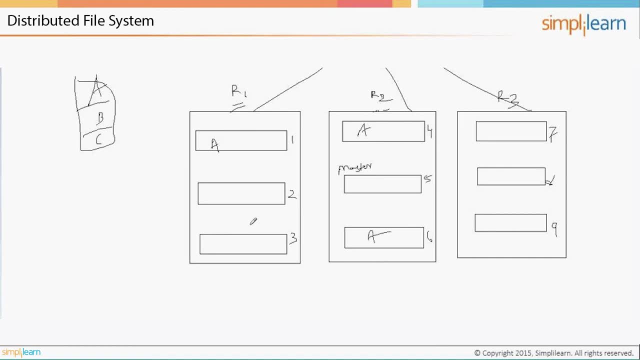 the same rack. it will always be installed in two different racks or multiple machines into different racks, basically right, so that even if one rack goes down, I will still have another copy available in another rack and then I can, you know, read the data. this is one of the you know feature of rack awareness. 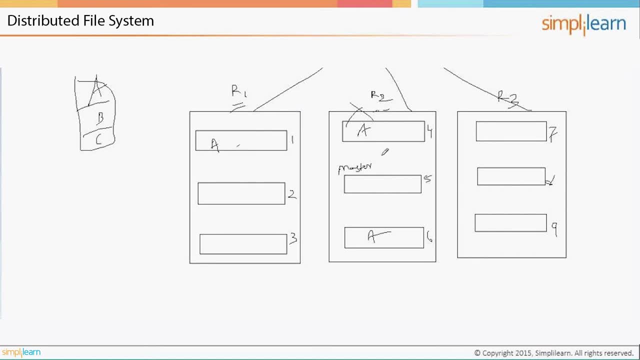 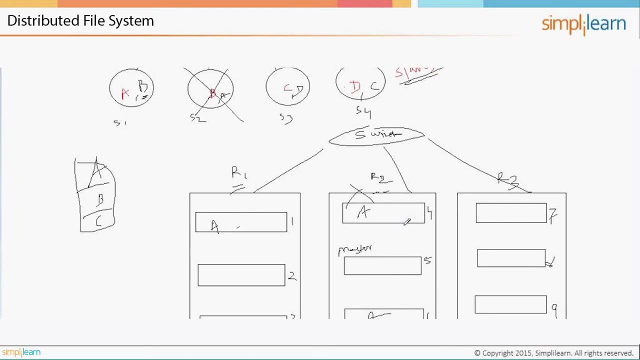 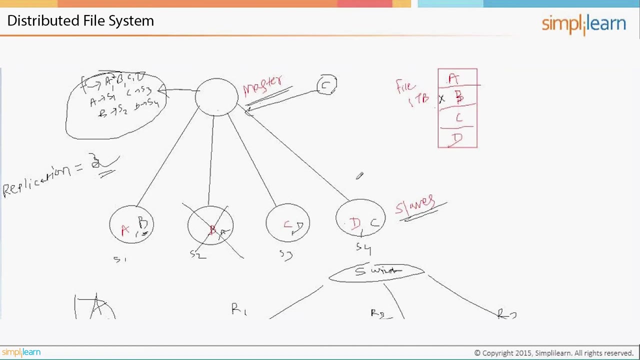 policy. there are other features as well, which we'll be understanding later, but I'm just explaining this because Hadoop supports this. Hadoop supports rack awareness and that's why it guarantees high availability of the data you know, even in case of rack failures. so that's why Hadoop is more reliable framework in. 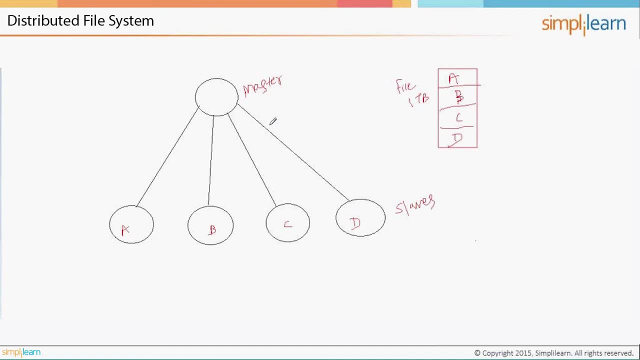 terms of availability and data sharing. and that's all about the Hadoop's task chance of the data. all right. so now let's talk about one other important difference between Hadoop and traditional system, which is Hadoop is faster in terms of processing the data. how so we will be understanding that. let's say, this file: 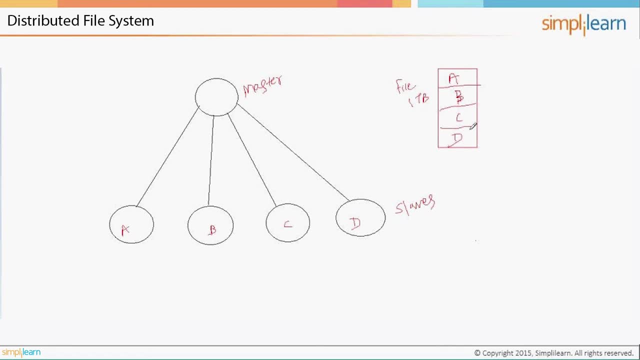 of 1 terabyte stored in distributed file system. we have ABCD blocks available in four slave machines. there is a client who wants to process the data, so he will submit a program to master. I am explaining you traditional distributed system approach. okay, how traditionally the distributed file system used to. 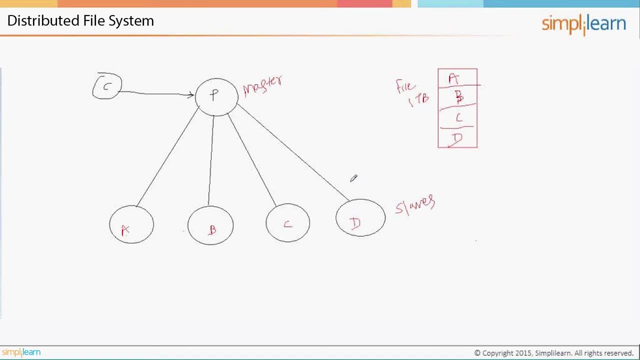 process the data first. so what? in traditional systems, what they used to do, they used to follow policy where, once the program is submitted to master, master will know the locations of the input data where it is stored. so what it used to do, it used to actually transfer all the data. 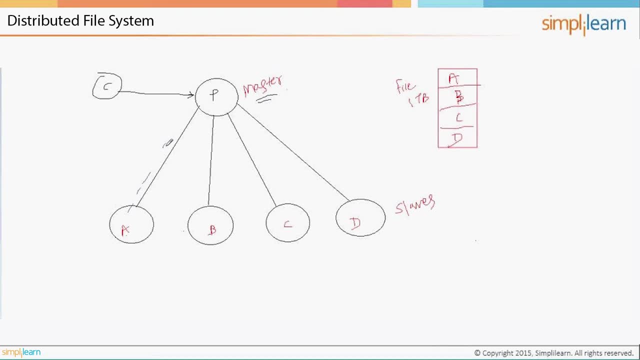 to the machine where program is running okay. so basically they follow a policy where data will be transferred to the machine where computation is running, where program is running okay- what used to happen? then it combines all the data and then program is using going to process the data. now there are couple of problems with this approach. 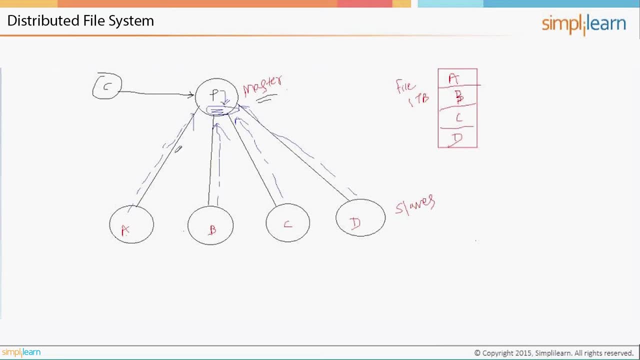 one is: if I am storing, if I am processing one terabyte of data, that means I am transferring almost one terabyte of data over a network, so it occupies lot of network bandwidth. that is problem number one. right, then you occupy all the data in one machine and then you are going to process it. so 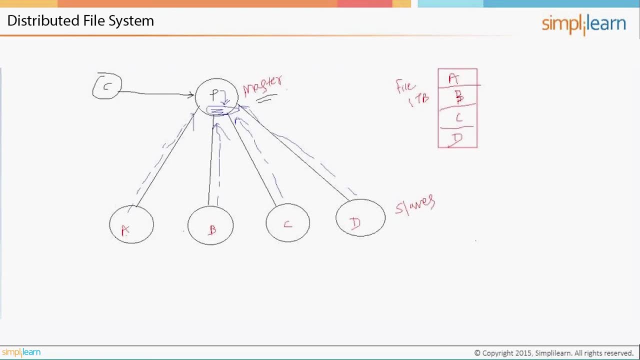 program is going to process that data, which means you are not really doing parallel processing first. first you occupy, occupy or bring the data from multiple sources and then accumulate it in one place and then try to process it. so that is not real parallel processing, and here we are also needing lot more. 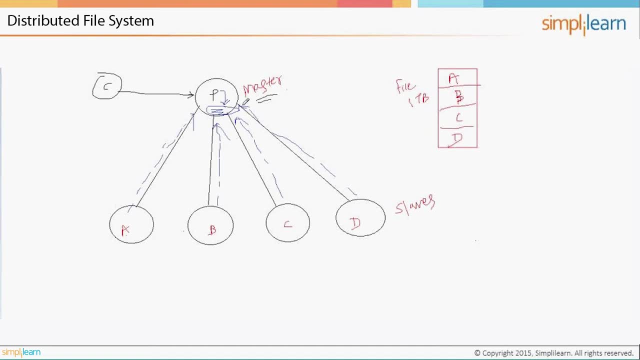 resources, CPU, RAM power- to basically achieve this computation in single machine. so these are couple of challenges with the traditional approach in terms of processing data. what Hadoop has done, it has actually done it everything in the reverse way. okay, so Hadoop is actually sending all the computations to the machine where 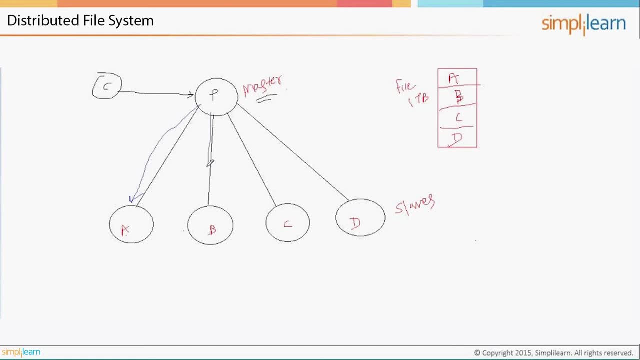 data is stored. so, basically, when the program is submitted to the master Hadoop, instead of sending data to the machine where program is running, it does the reverse way: it sends the program to the machine where data is stored. so it does data locality operations and it basically sends programs to those machines where 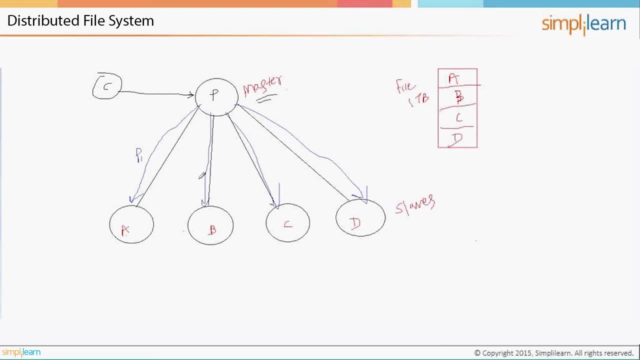 individual block of that file is stored, so it creates multiple instance of the programs and they will be basically sent to different machines to process that. so P 1 is going to process a, P 2 is going to process B, P 3 is going to process C, P. 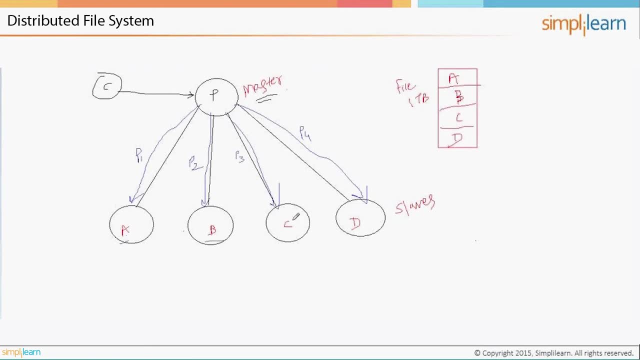 4 is going to process D, and all of them are parallelly processing individual block of this file. okay, and they are generating intermediate output: output 1, output 2, output 3, output 4 and so on, so forth. okay, now, what are we doing here? what are the advantages in this approach? we are first: 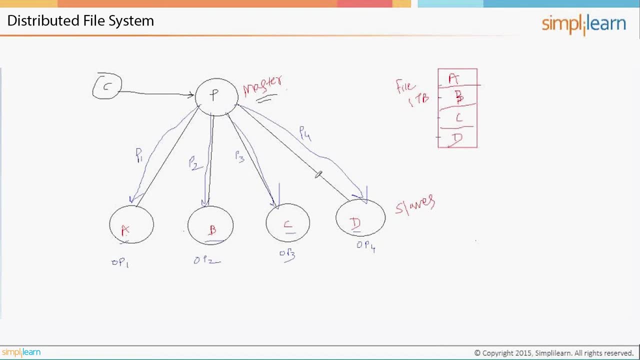 of all avoiding entire net data transfer over a network. so we are saving lot of network bandwidth. we are just transferring program so it doesn't occupy much network bandwidth and we are actually doing parallel processing. each blocks can be processed independently and parallelly for that file and then 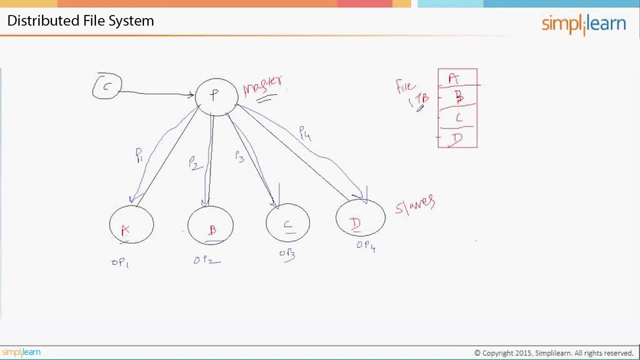 respective output is being generated after processing that data right now. this step is going to be generated after processing that data right now. this step is going to be generated after processing that data right now. this step we are not yet done. this is just an intermediate output. after that, what it? 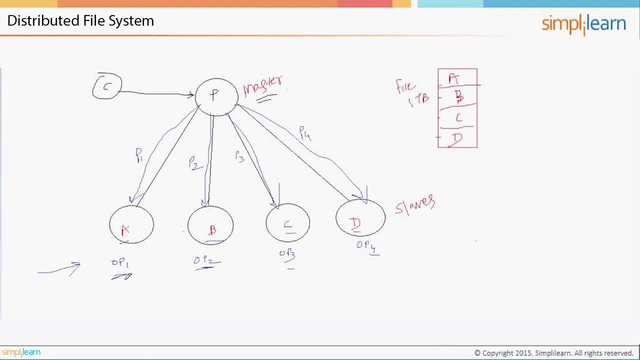 does? it actually combines all this output which is generated by every stage, and it tries to merge them together and then send it to one of the machine where it runs another process called reducer, with process this data and then generate the final output. okay, so this is how Hadoop processes the date. again, I have 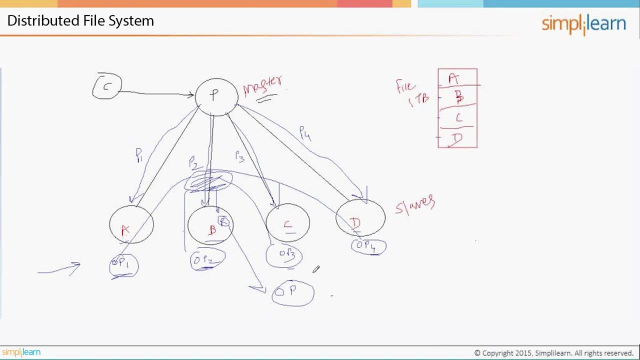 explained you a very high level over you of what we are to process, because we do not test it, but it is generally understandable and it is never textable also. so this is how Hadoop does that listening helps of what Hadoop does in terms of processing the data. we will understand. 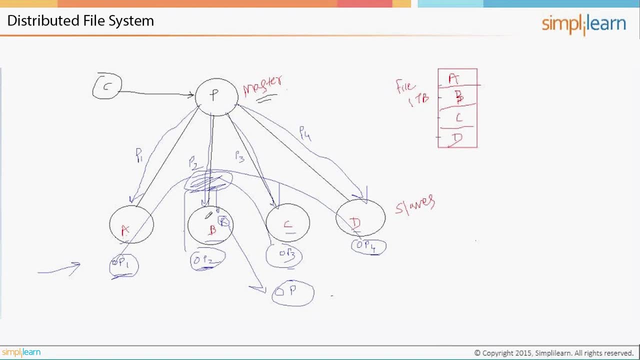 it in detail when we talk about MapReduce. but this concept, this, you know the way of processing this data- is referred as map and reduce. so this is called MapReduce and it follow one very important design pattern which is called divide and conquer. so map is divide and conquer is reduce. 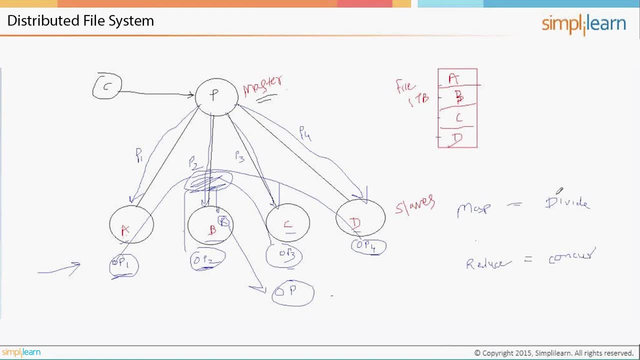 okay. so divide means what you have a big problem to solve. you first divide that problem into smaller chunks and then independently and parallelly process those smaller chunks first. once you get the output- intermediate output- you combine them and then process it one more time to generate the final output. 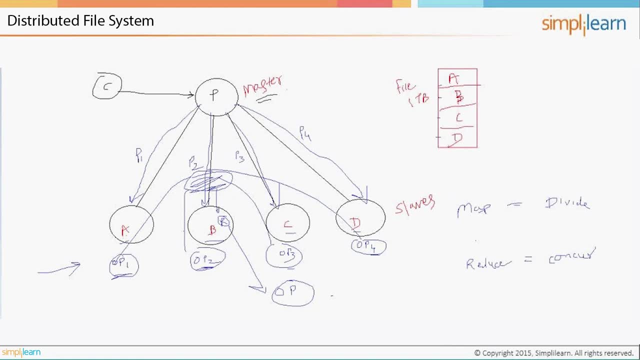 that's the fundamental concept that lies behind map and reduce. ok, and with that concept, with that approach, it is actually achieving parallel processing and it is processing the data 10 times faster than the traditional distributive system. so this is also one more important advantage that hadoop provides in terms of processing the data using map and reduce. 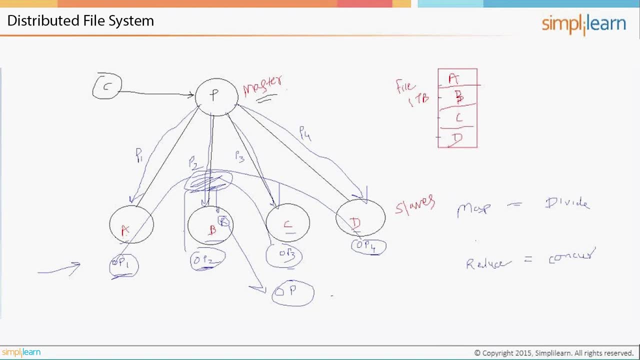 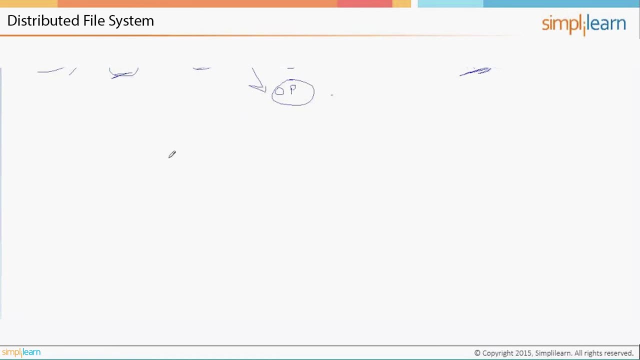 that also made it more faster. what is exactly Hadoop? is it a database or not? so Hadoop is basically a framework which helps you to achieve two important things. we have talked about big data, and we already understood that if you want to process big data, you have to. 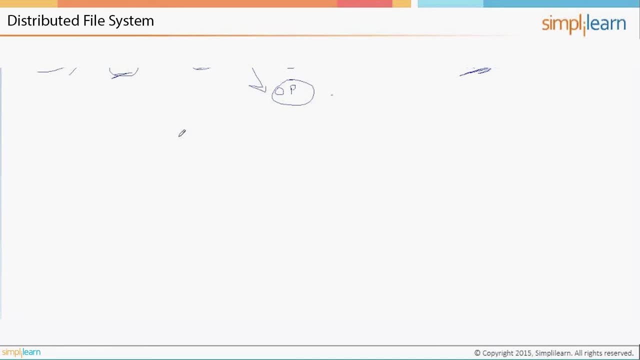 first store it somewhere in a distributed manner and then you can parallel process it. so Hadoop is a framework which gives you this capability. it has a capability to store big data in a distributed and efficient way using a component called HDFS- Hadoop distributed file system- and it has a 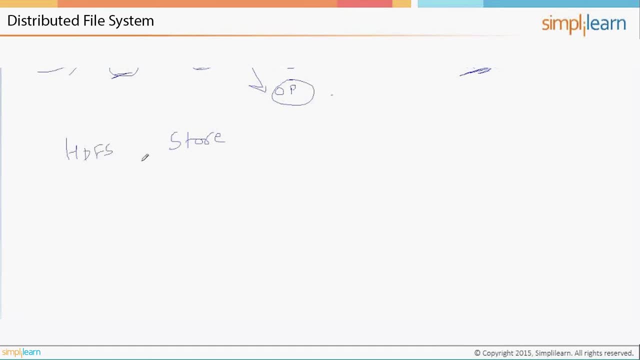 capability to process your data. once you store it on HDFS, you can process it parallelly using MapReduce. so these two components together forms your Hadoop. so Hadoop is a framework which gives you these two capabilities using these two components. that's how you should remember the definition, so that you 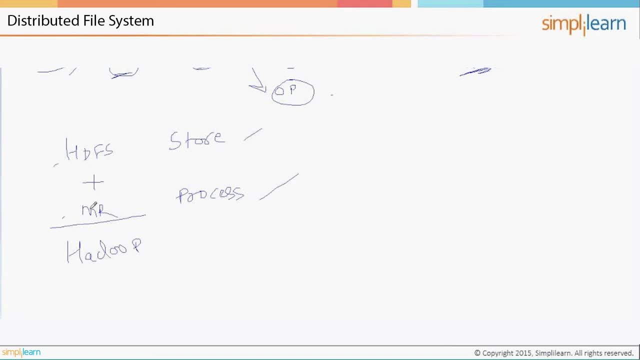 will never forget what is Hadoop. okay, and you also have some of the. I mean one more component which is a Hadoop, so it is a Hadoop, so it is a Hadoop, so it is a component in latest this thing which is YAN, latest Hadoop version. YAN is a. 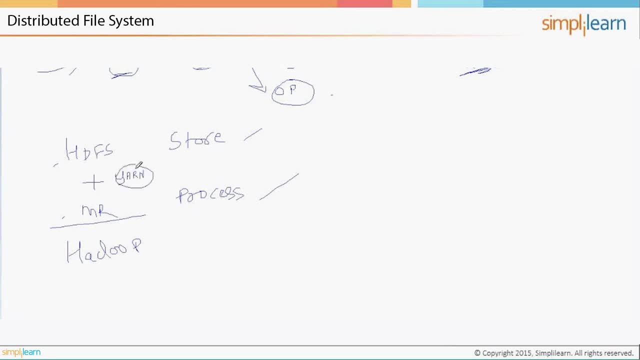 cluster resource manager. we'll talk about it later, but yeah, YAN is is a recent addition to Hadoop latest versions. all right, have a great day ahead, thank you.